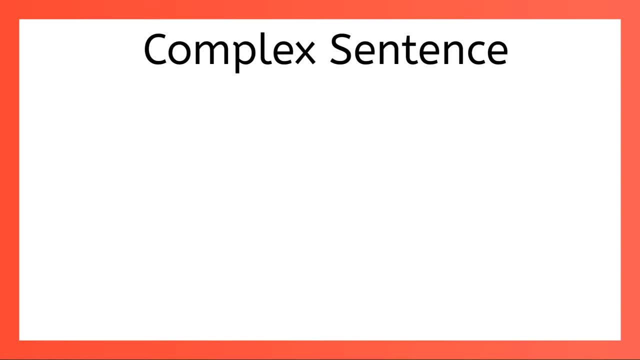 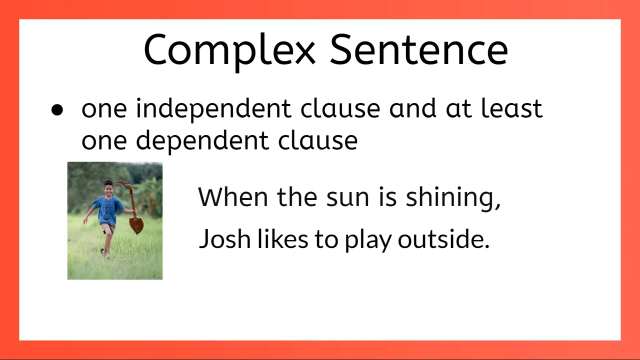 all very important in understanding complex sentences. A complex sentence contains one independent clause and at least one dependent clause. So we could have a simple sentence, like Josh likes to play outside, and we could add a dependent clause to it, like When the Sun is shining, and voila, we have created a sentence. It has one independent. clause and at least one self-dependent clause to it, like you see here. After that we have six and one dependent clause and the subordinating conjunction when, In this complex sentence, the dependent clause comes first before the independent clause. When the dependent clause comes first, it must be followed by a comma, because we are 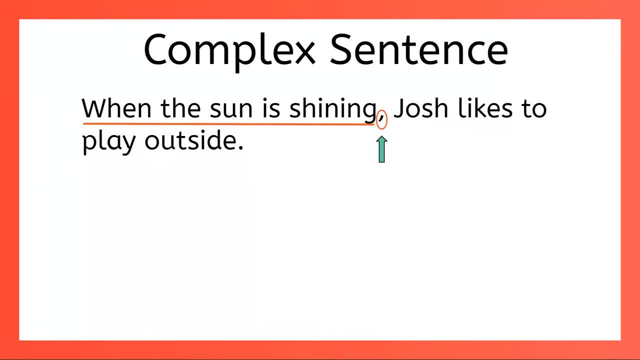 placing it before the subject of the sentence, In this case Josh. However, the dependent clause can also be placed after the independent clause, And when that happens, no comma is needed. Read with me: Josh likes to play outside when the sun is shining. 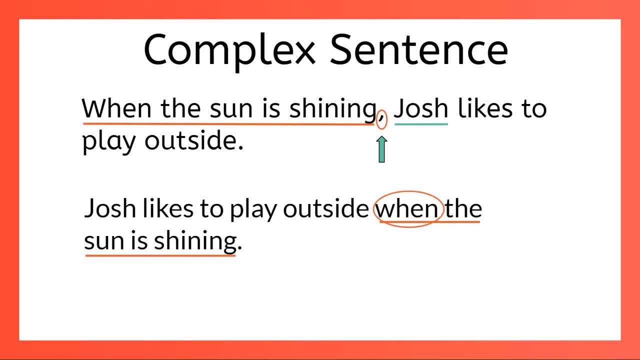 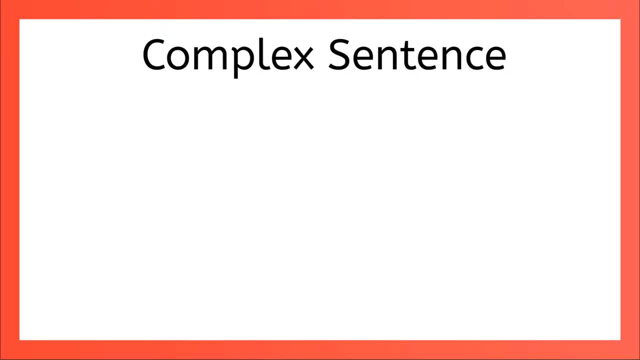 We still have our dependent clause, but it comes after the independent clause, so there is no need for a comma here. Okay, Let's make a complex sentence. Remember it will need a dependent clause, like: If I prove that I am responsible. 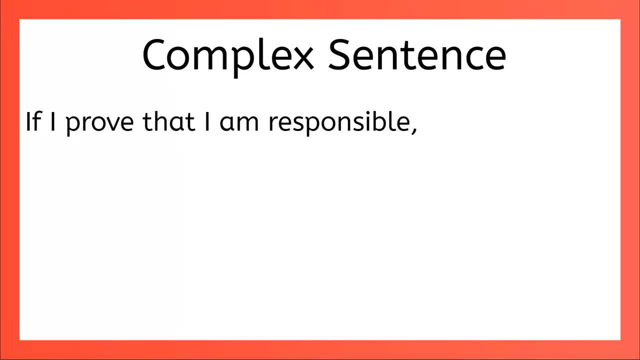 That's a dependent clause because it has a subject and a verb and it begins with a subordinating conjunction. If we add an independent clause, we have a complex sentence. If I prove that I am responsible, my parents said we can get a puppy. 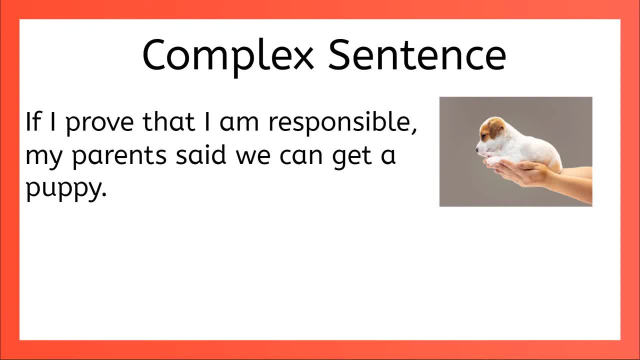 Okay, How cute. Since the dependent clause comes first, we add a comma, but we can also reverse the order of the clauses and no comma is needed. like My parents said, we can get a puppy if I prove that I am responsible. 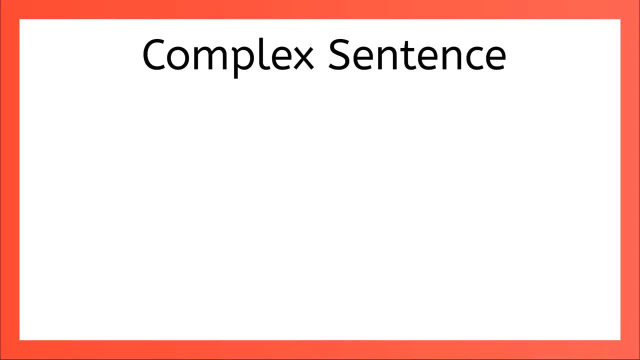 Let's try another complex sentence. We'll start with the dependent clause. How about Because? Because it was raining? It has a subject and a verb, but the subordinating conjunction, because, makes it a dependent clause. What's an independent clause we could add to form a complete sentence. 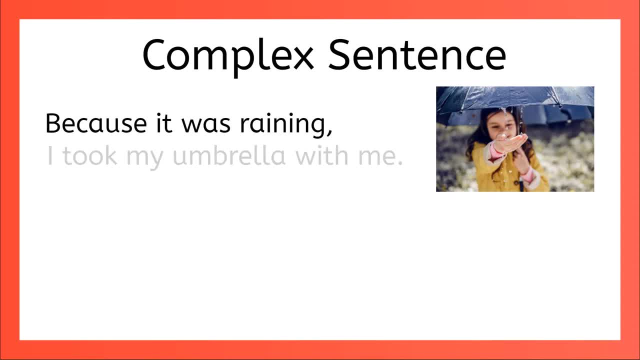 Maybe Because it was raining, I took my umbrella with me. Since the dependent clause comes first, we add a comma. But remember, we can reverse the order of the clauses. I took my umbrella with me because it was raining And this time no comma is needed. 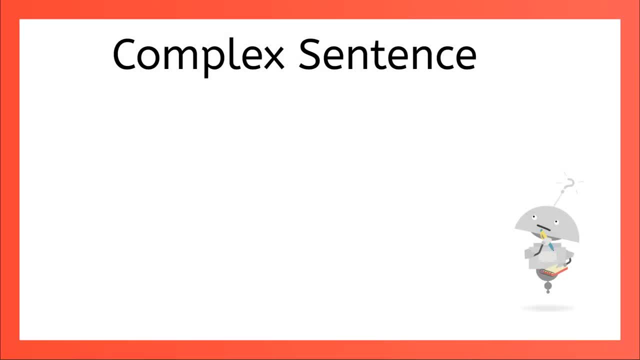 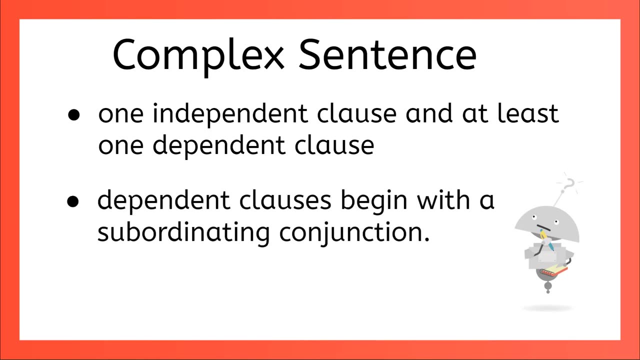 So now you know what a complex sentence is. Complex sentence contains one independent clause and at least one dependent clause, And you can always spot those dependent clauses And you can always spot those dependent clauses. And you can always spot those dependent clauses Because they begin with a subordinating conjunction. 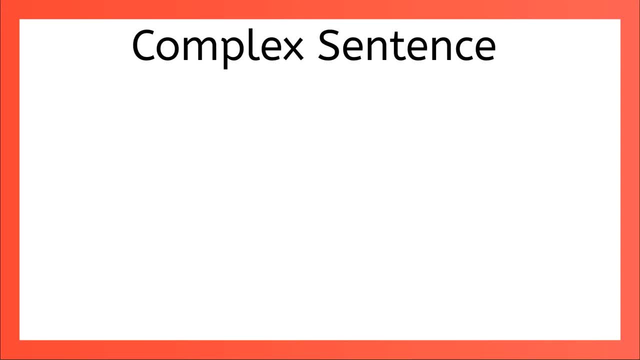 Some sentences are tricky and at first they look like complex sentences, but they're not. For example, Before lunch I always wash my hands. We have an independent clause- I always wash my hands, But Is before lunch a dependent clause. 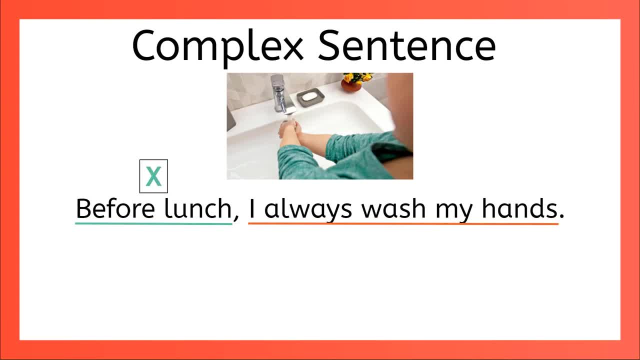 Nope, It is not a clause because it doesn't have a subject and a verb. So before lunch is a phrase, A propositional phrase to be exact. This sentence only contains one clause, so it's a simple sentence. However, if we change that phrase to a clause with a subject and a verb, that simple sentence. 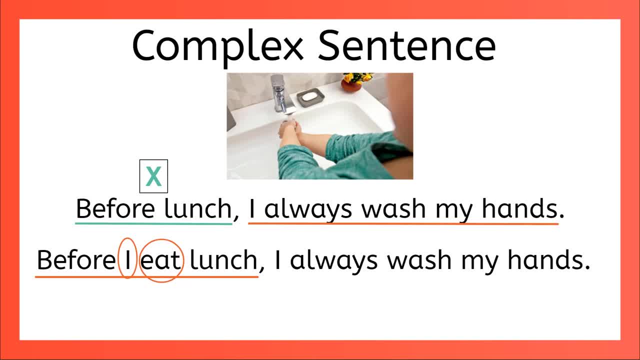 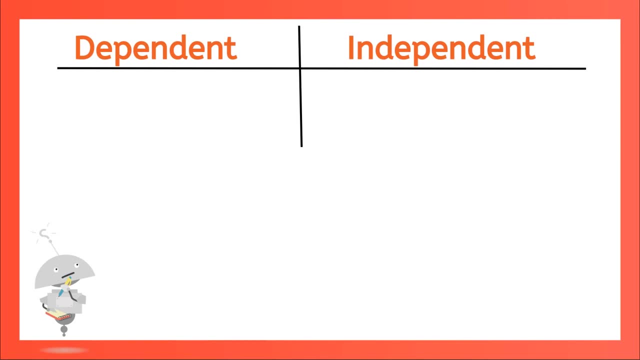 becomes complex. Before I eat lunch, I always wash my hands. Now we have a subject and a verb, so we definitely have a dependent clause. Let's build our own complex sentence. We'll start with a dependent clause. It'll need a subject and a verb. like Mia listened. 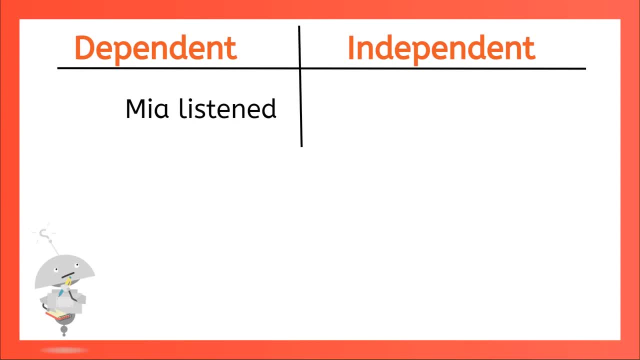 And then it will need to begin with a subordinating conjunction. Mia listened. How about, as Let's think of an independent clause, Something that might have happened? as Mia listened, Maybe she learned new things. If we join the dependent clause with the independent clause, we have a complex sentence.